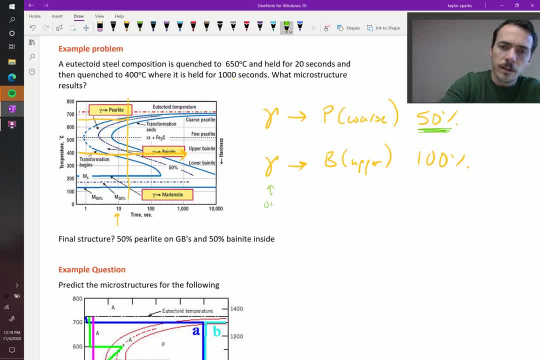 So this to start with. we only had 50% to start with because we'd already converted 50% to coarse perlite. So we did a 100% conversion of 50%. So our final microstructure is going to be perlite 50% and bainite 50%. Now you might ask: well, when we held this down? here. why wouldn't the perlite turn into bainite? Perlite cannot turn into bainite because perlite is big, thick grains And if you hold it for any it's never going to form smaller grains because that's increasing its surface energy penalty. So, if anything, things want to coarsen. 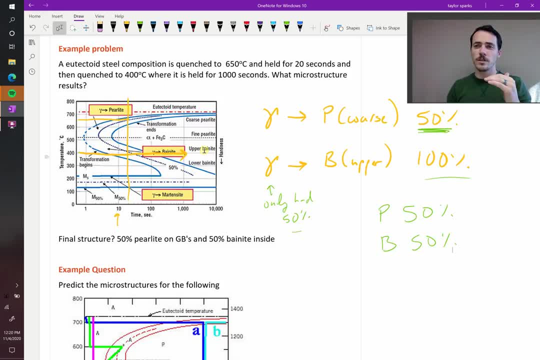 but if you did the bainite first and then you did the perlite, all of your bainite would start to turn into perlite because it would coarsen. But you'll never go the other way. It'll never. 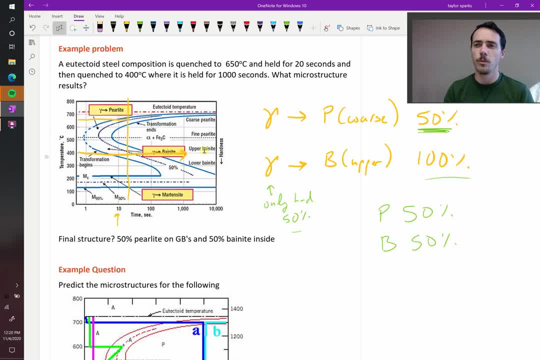 start from really thick grains and all of a sudden get smaller ones, right With the heat treatment. you have to do something else to make that happen, right? So that would be our final structure: 50% perlite on the grain boundaries and then 50% bainite on the inside, And that's. 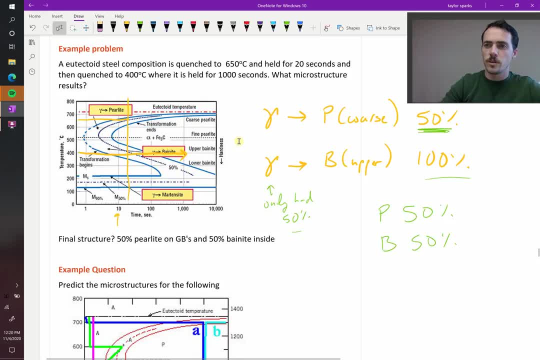 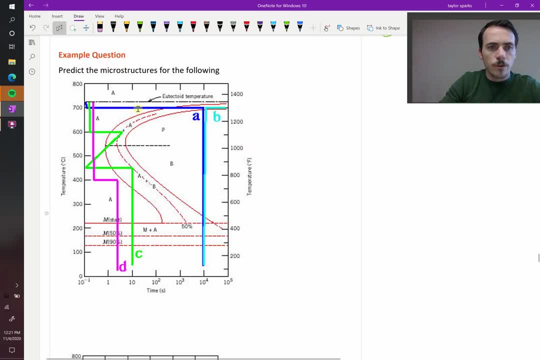 just because it's going to form along the grain boundaries first, That's going to be the first thing that gets consumed, right? How about this one? All right, let's do number A Right. A is this dark blue line where we hold it for a long time? To me it looks like maybe. 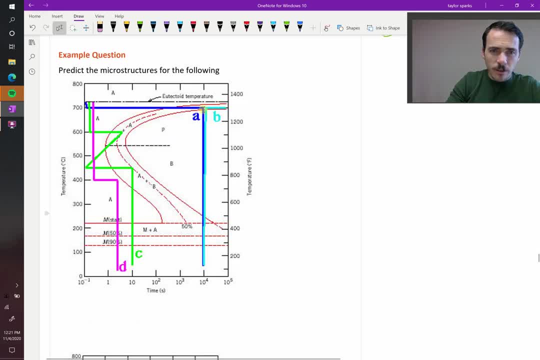 past 50%, maybe 75% of the way or so, and then you quench it down through this martensitic transition. So for A, what I would expect from this, you know- not great drawing- I would expect for A that you have maybe 75% perlite and 25% martensite. That's what I would. 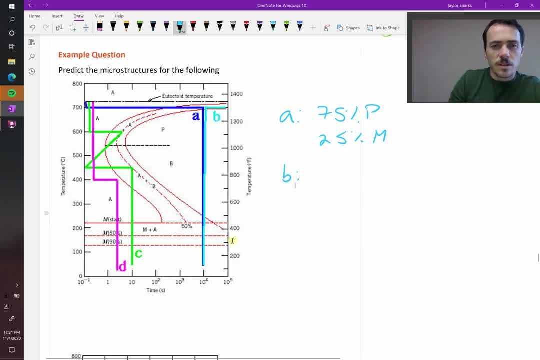 expect Now B? how's B going to be different? B is the exact same as A, except then we heat it up and we hold it for some long amount of time. So then we're going to get 100% spheroidite. So you might say, why don't you get 100% tempered? 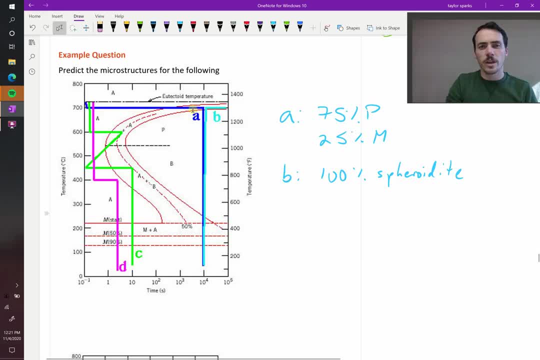 martensite or something. The reason why is because if you're holding anything at really high temperature for long enough, all of your lamella, all of your things, like your tempered martensite, which is coarse, you know dispersions, they're all going to coarsen, right, You're giving? 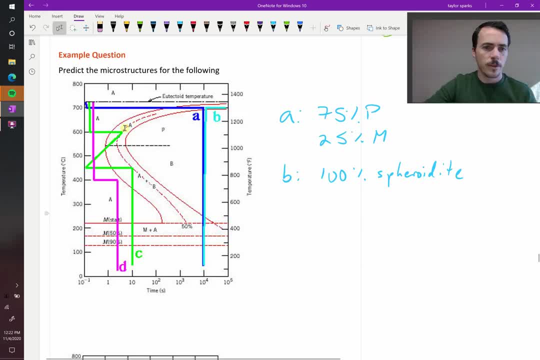 them enough thermal energy that it's going to end up as spheroidite. What about this one C? C goes down to 600.. You hold it to the 50% line, Then you bring it down here and you reset it. 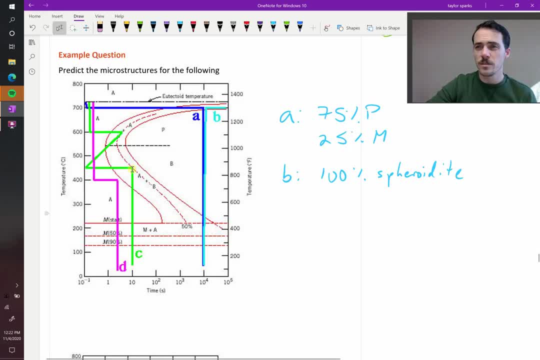 And now you hold it for that amount of time- 10 seconds- and it reaches the 50% line there, And then you quench it. So what do you end up with for C? C is going to end up with the following. It's going to be 25% perlite, or, sorry, 50% perlite. It's going to be 25% bainite, which is again 50% of the remaining 50%, And then it's going to be 25% martensite. 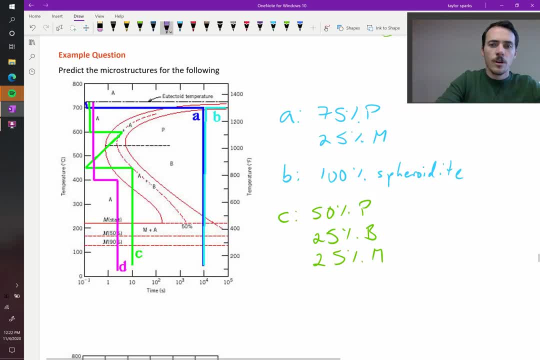 Right. So that's what we end up with there. What about D For D? we now have that, we quench it and we hold it out to here, but since it never touches that line, we never start forming bainite, And 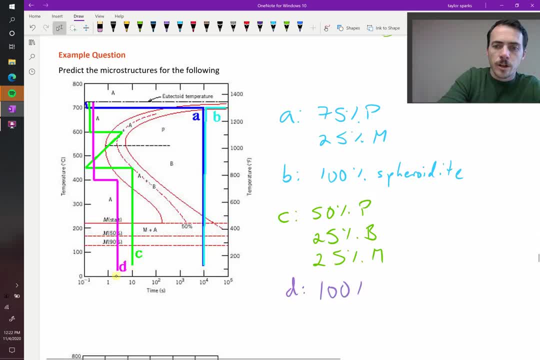 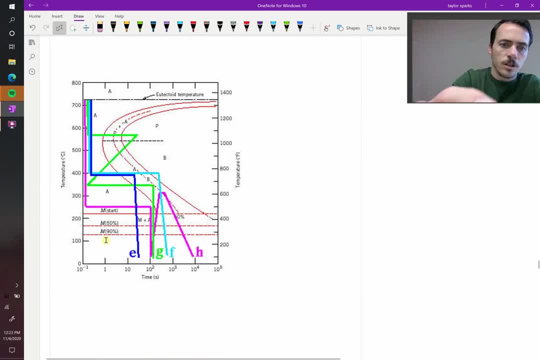 then you quench it straight down, So you end up with 100% martensite. All right, Let's do a couple more. How about this one over here? So we're going to do E, F and G. All right, E, they quench it. 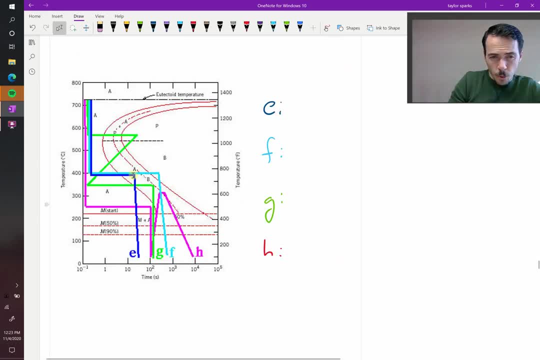 past the nose and then they hold it to about 25% bainite. So we're going to do E, F and G going to have 25% bainite and then they quench it down, so the rest is going to turn into martensite. 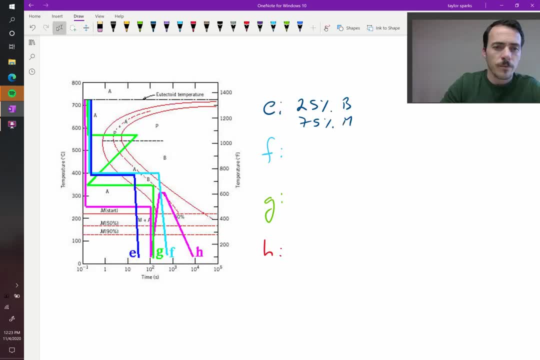 so that's going to be 75% martensite, everything that was left over. F. they hold it all the way through here to bainite and then they quench it down, so it's going to be 100% bainite. It's not. 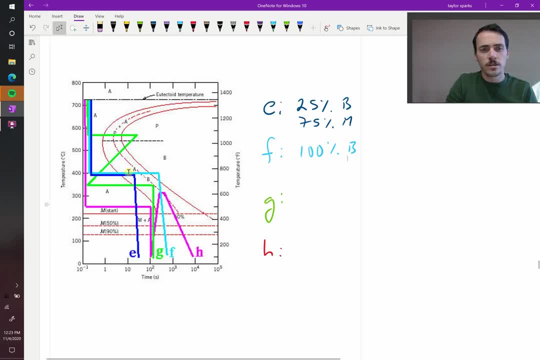 going to have any martensite because we consumed all of our austenite turning into bainite and you only get martensite from austenite. so if you've consumed all of it, it doesn't matter that you quenched it. you don't get it All right for G. we're going to get 50% bainite and then we're. 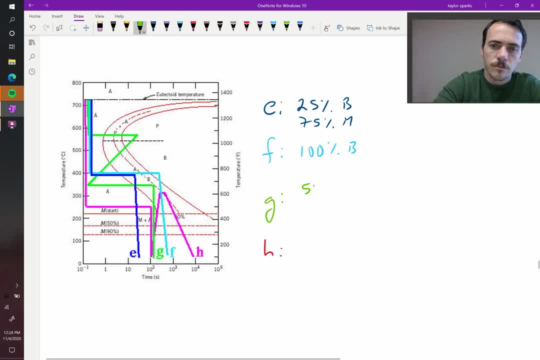 going to quench it. so we're going to get 50% martensite and then H they hold it down to here. they now hold it at this temperature. just before it touches the line they quench it. so now you have pure martensite, 100%, and then they heat, treat it up to this relatively low temperature for a while. 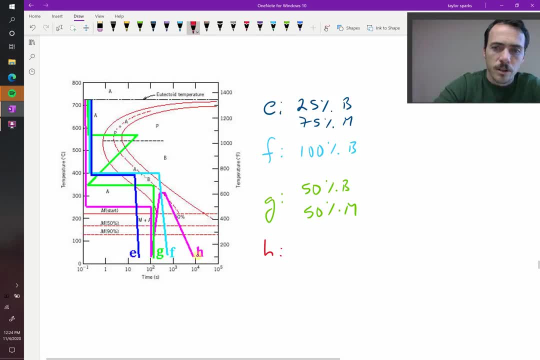 and then they bring it down. That is a recipe for tempered martensite. So we're going to get 100% tempered martensite. So that's how you use these TTT diagrams to predict the microstructure of steel and again, since we know the properties of these things, martensite.